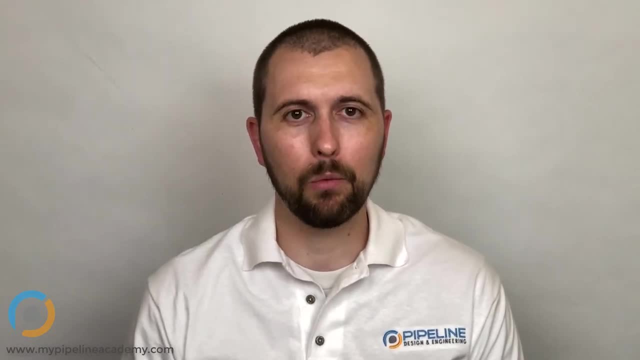 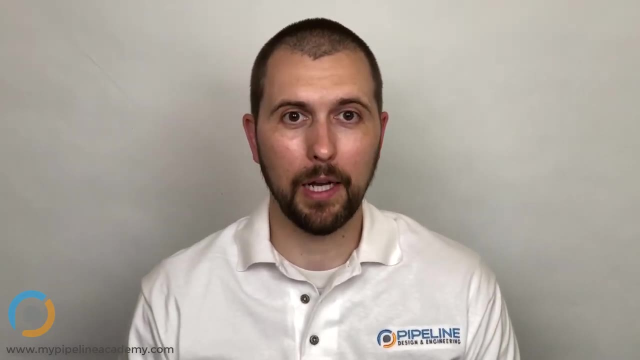 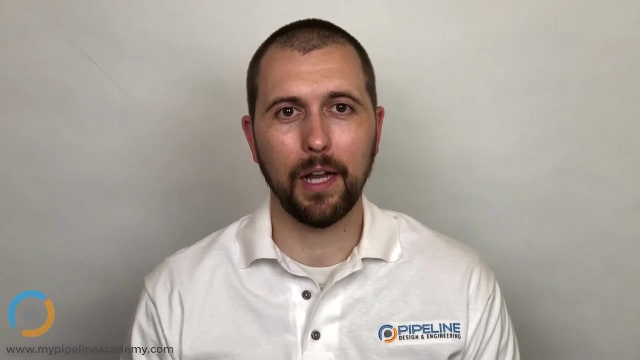 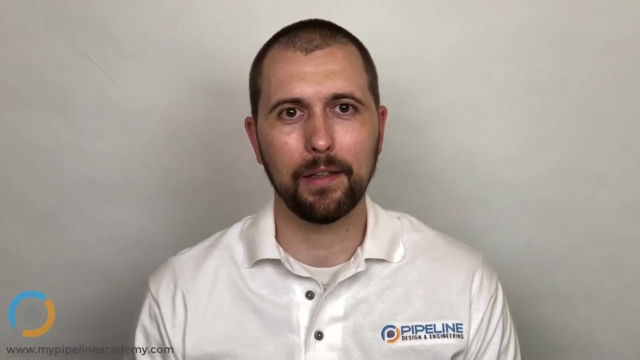 protect or hide what's on the inside of that part. One of the most common and a very reliable method of joining two parts together is screws or fasteners. There are a lot of different types of screws and fasteners and they're great. They work very well, They're time-tested. They're just a really solid solution to join. 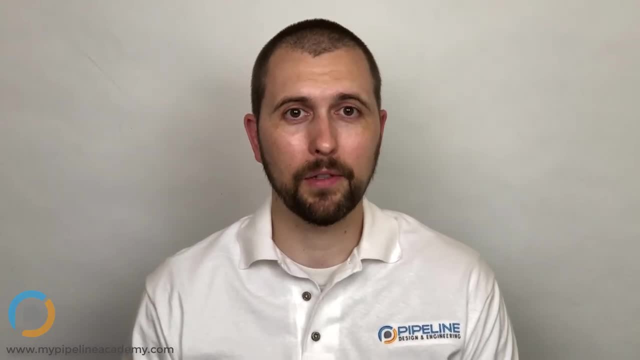 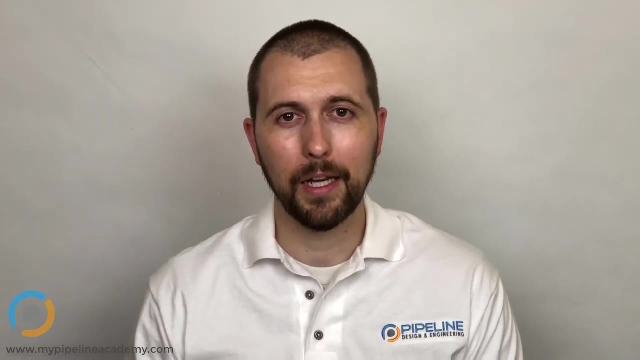 two parts together. One of the downsides with using fasteners is they become an extra part. So instead of just buying the two parts that you need to join now, you need to buy the fasteners as well, And then it's going to take someone- someone working on the assembly. 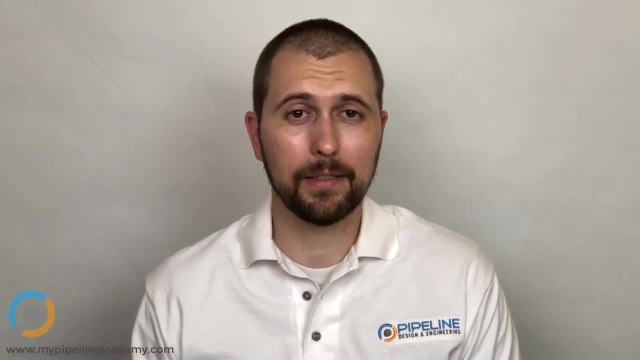 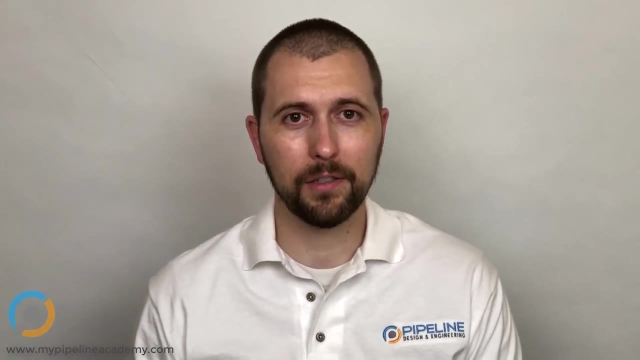 line to actually install those fasteners And, granted, it doesn't take a lot of time to do that, but it takes some time. So the added cost of the material of the fasteners and the labor involved in installing them, that adds a little bit of cost to your product. 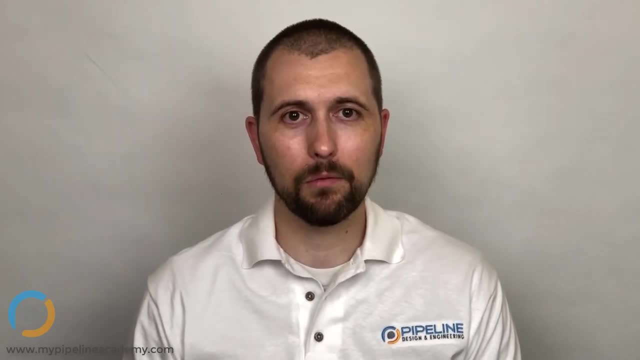 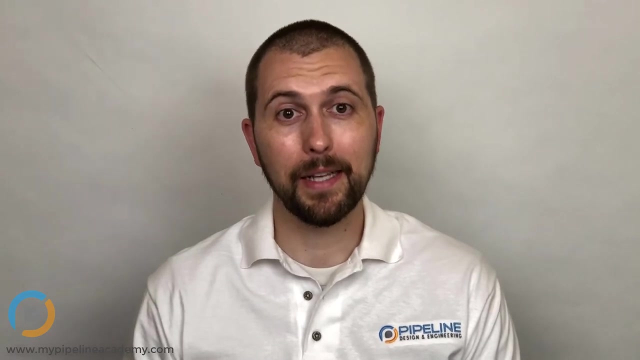 So in that sense they're not ideal, But they are really good. Thank you. They're really great tools to use for joining two parts. Another method of joining two parts- and this works well in plastic parts but not so well in metal parts- is using snap pins, or what are called gripper pins, And we won't get 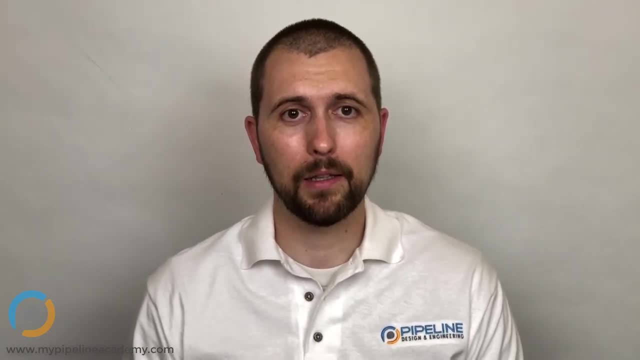 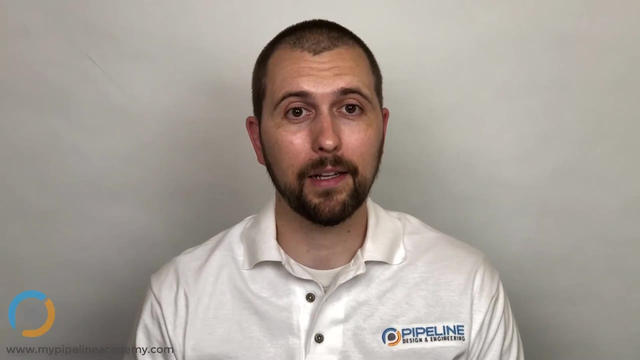 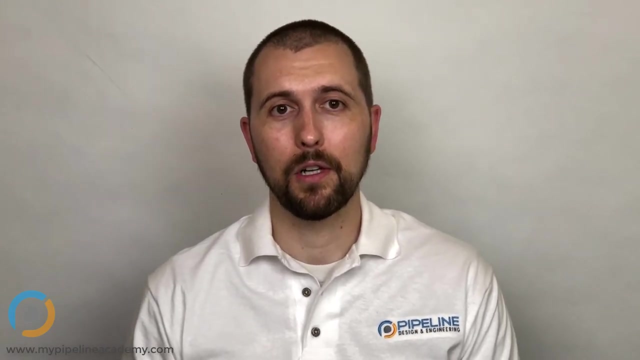 too much into the details of what those are, but they rely on the soft kind of malleable, flexible nature of plastic And they allow the two parts to be joined together without the use of any additional hardware such as a fastener. 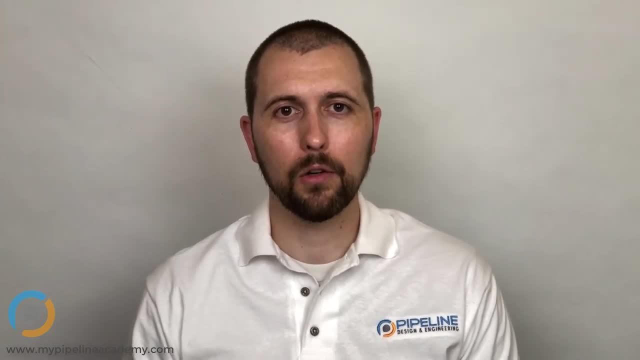 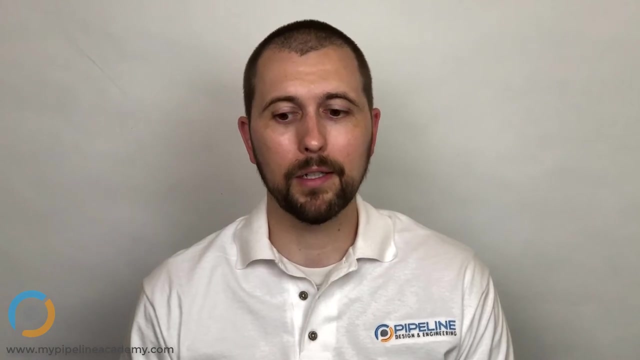 That's kind of the strength of using snap features or gripper pins in your molded plastic parts is that they don't require any additional tools or hardware. They're features that are built directly into the parts themselves and allow the two halves to be joined together. 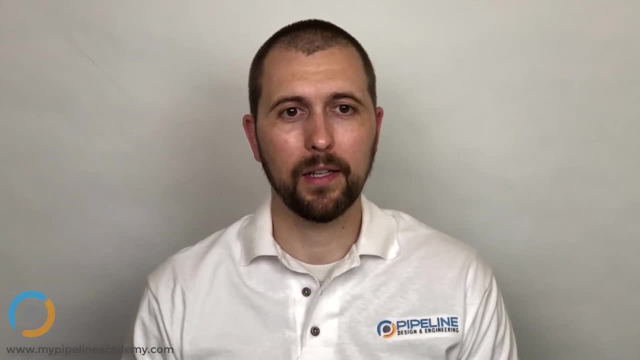 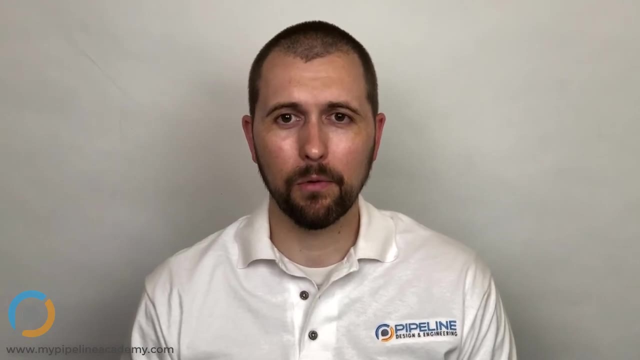 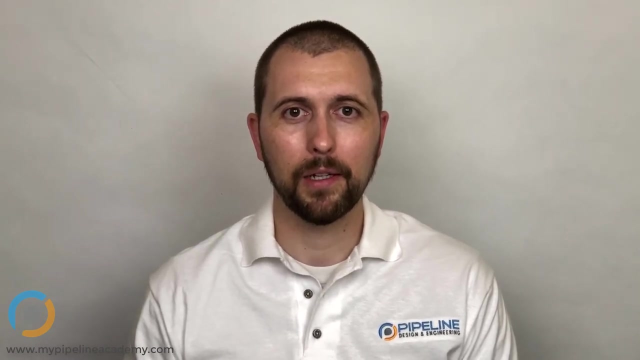 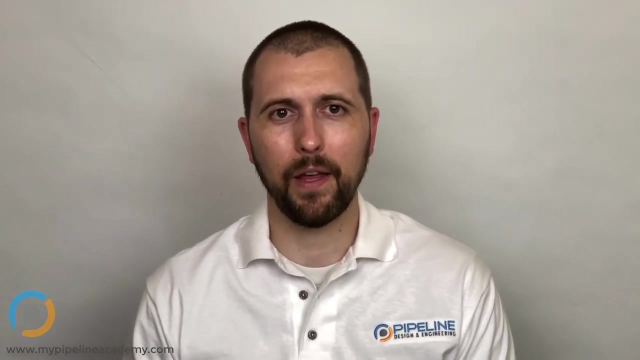 A press fit. Yes, A press fit fit is another joining method, and a press fit relies on usually well, very tightly controlled tolerances and an interference between, like a pin on one side and a hole on the other side, and we'll get a little bit more into the details of that in some of our written literature. but 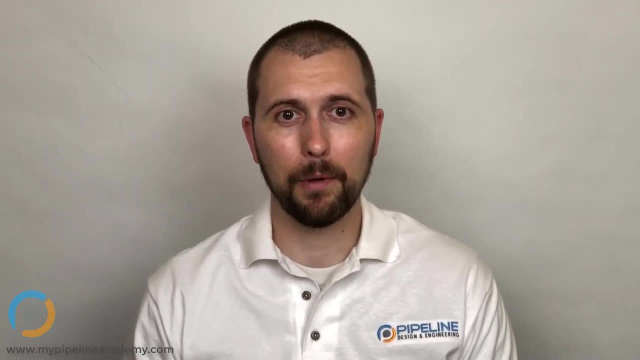 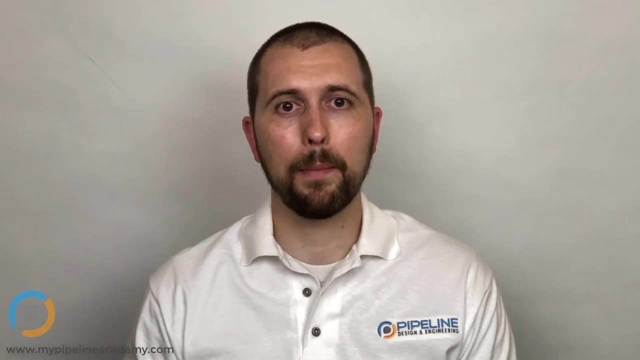 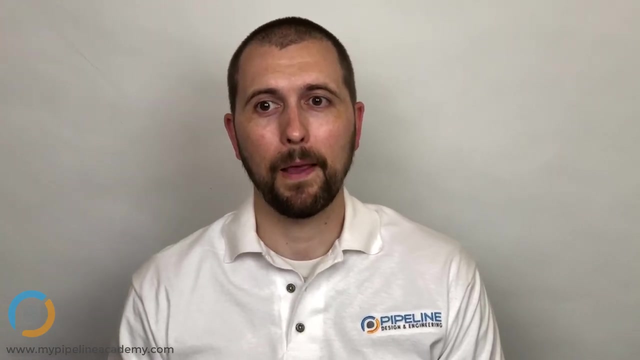 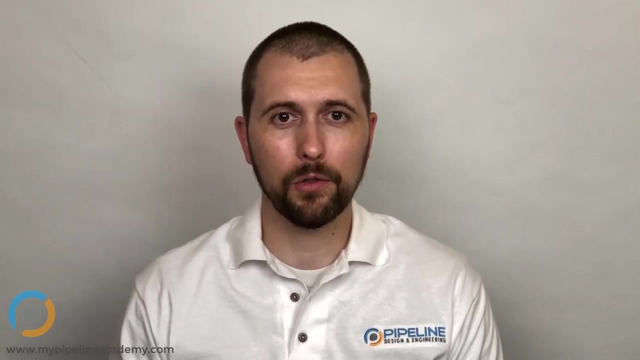 a press fit is a very common method of joining two parts together. ultrasonic welding is a common process that's used. it's maybe not as common as just using screws or snap features or a press fit, but ultrasonic welding definitely is a process that you can use to join certainly two plastic. 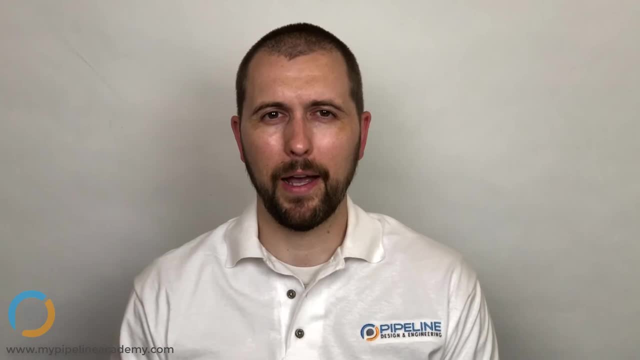 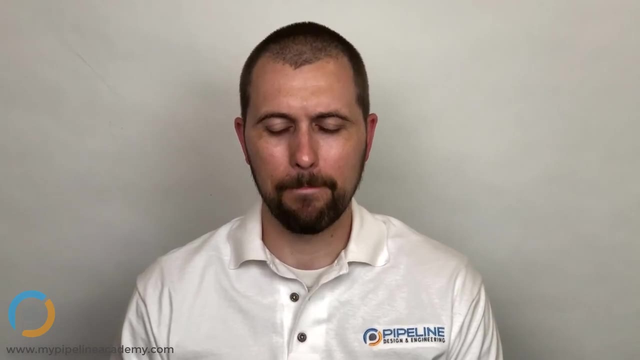 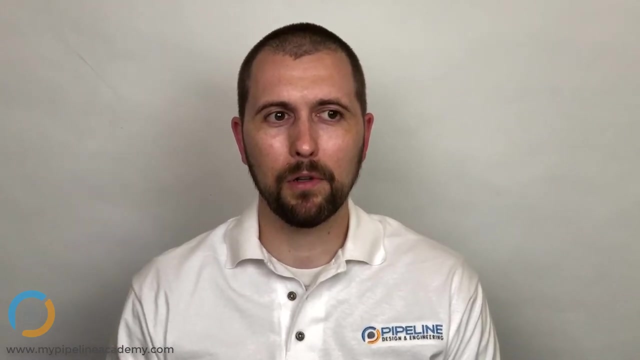 parts. that's probably where it's most commonly used. i have read here and there that it can be used on metal parts, but i'm not really very familiar with that application. adhesive is something that can be used. a note on adhesive: a lot of people, especially people who are not really familiar with the field of product. 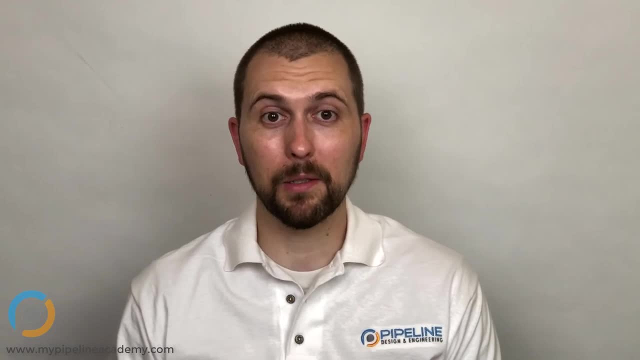 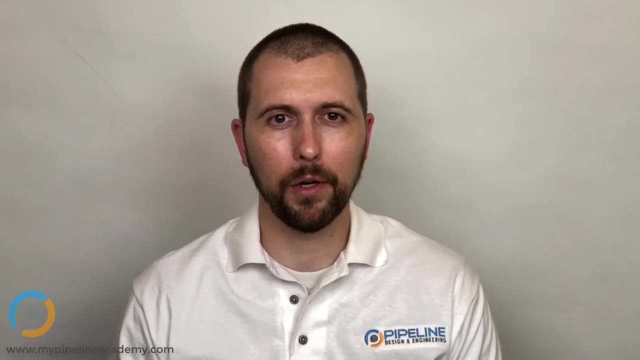 development might go directly to adhesives because it, you know, seems simple: right, just apply some adhesive and push the two parts together and boom, you've got your parts joined. well, you, you. in reality, adhesives are fickle and most product designers don't like using adhesives because 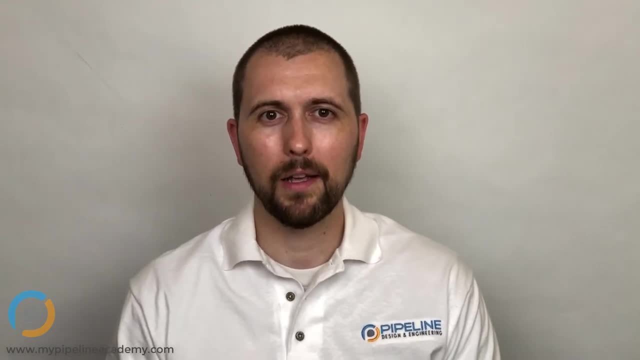 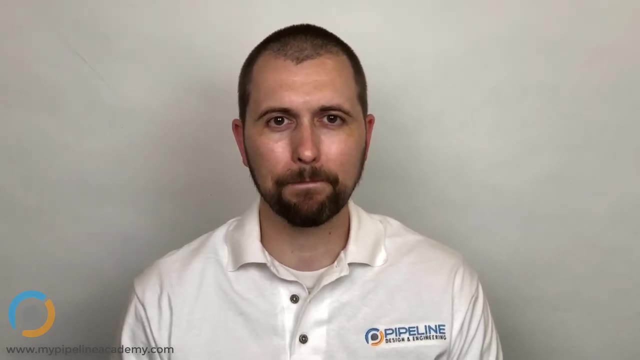 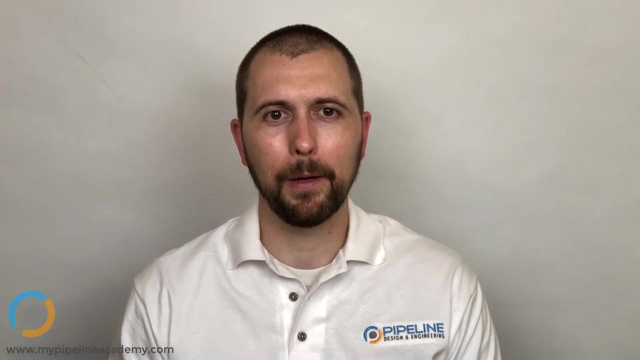 they're fickle, it's hard to get it just right, it's hard to make the process of applying that adhesive perfectly consistent from you know part to part. so yeah, adhesives they're. they're somewhat common and they're certainly used in industry, but a lot, of, a lot of product designers, including myself, don't like using adhesives. 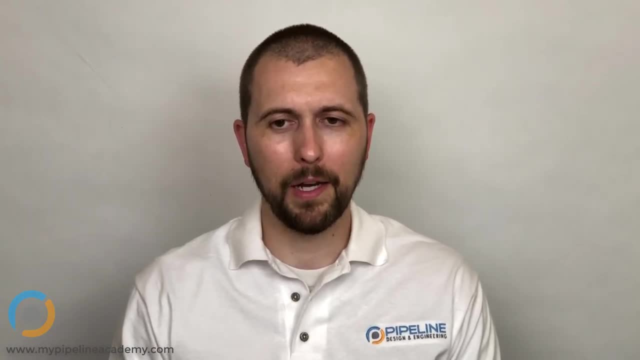 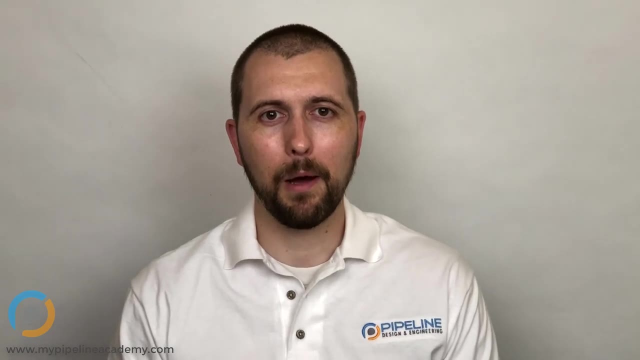 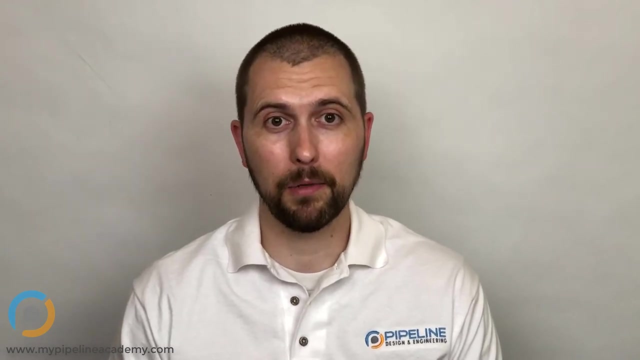 because they're fickle, and then one of the last processes to talk about is is just tape and we're not talking about, you know, like scotch tape. we're talking about more industrial tape. 3m is a big company and they make a lot of products, but some one one category of products that they make. 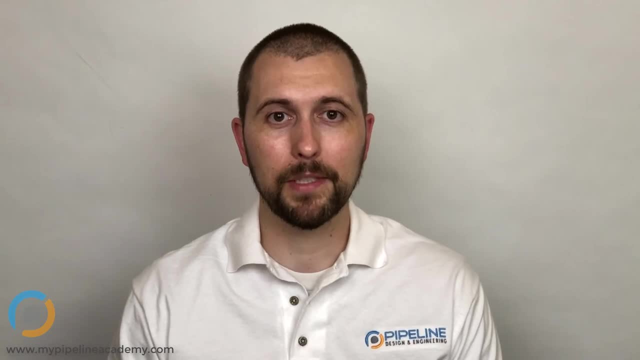 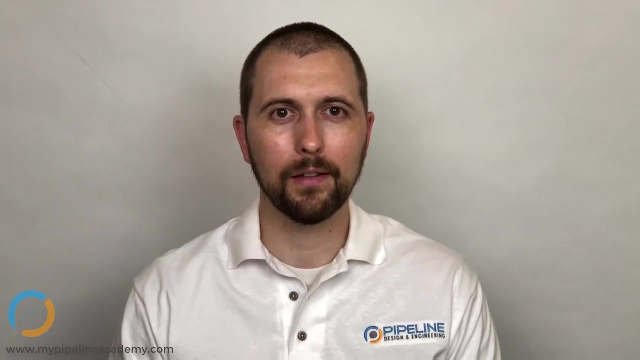 very well are industrial adhesive industrial tapes, sometimes referred to as transfer tapes, but these are very, very strong adhesive tapes that will allow you to bond two parts together. so, as a mechanical designer, it looks like i have two options that are pretty good. one of them is fasteners like screws, and the other one is, uh, the gripper pins, perhaps. 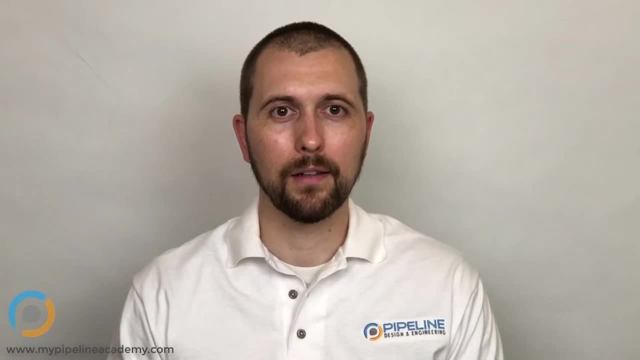 so i'm thinking about the pros and cons of both of these. and if i'm going to do the gripper pins, i have to put them in the cad model. so it takes time, more thought. but if i'm doing the screws, the fasteners, all i gotta do is basically just put a hole in the cap and that's it. 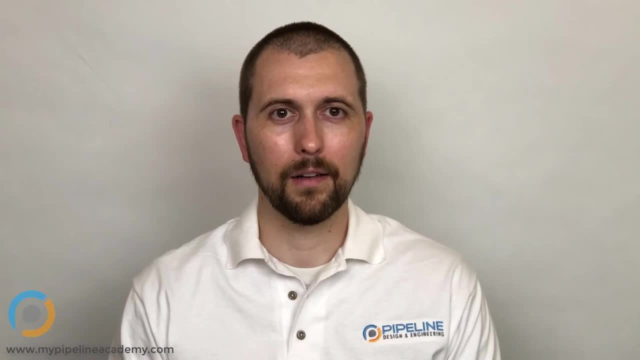 hole in the cad model and i'm trying to weigh out in my mind when should i use each one? sure, yeah, um, so one one point is that you typically do add your fasteners to the cad model as well. uh, there are a few reasons for that, but for now we'll just say it is good practice to put. 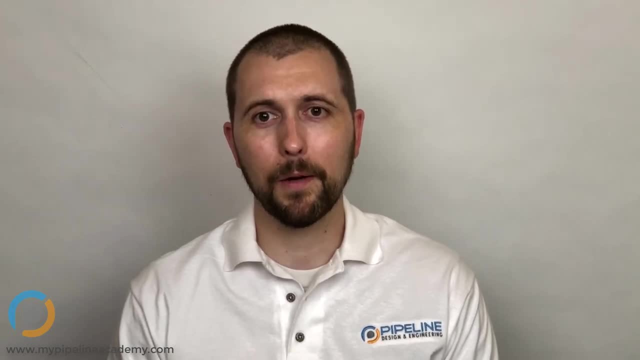 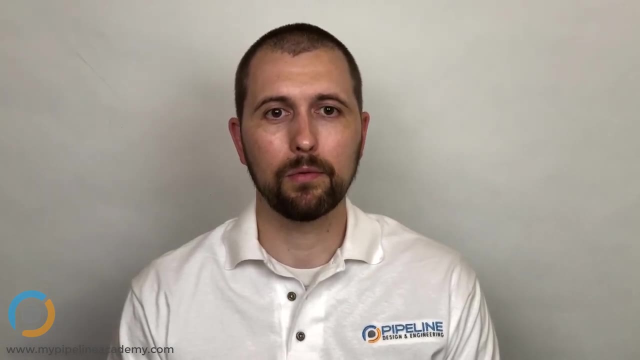 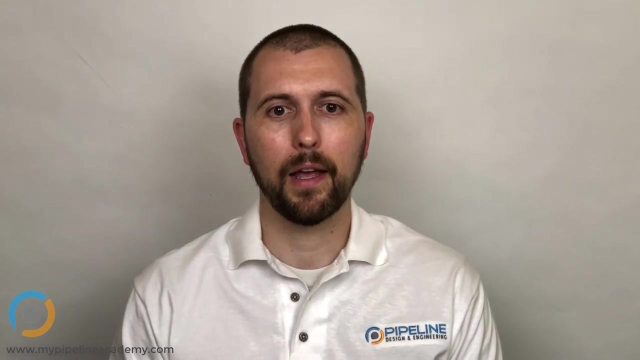 fasteners in your cad model, so you don't really save any time there. um, i think the the big difference between using screws or gripper pins is is one: gripper pins only work for plastic parts. you wouldn't use gripper pins in in metal parts. and and the other thing is that 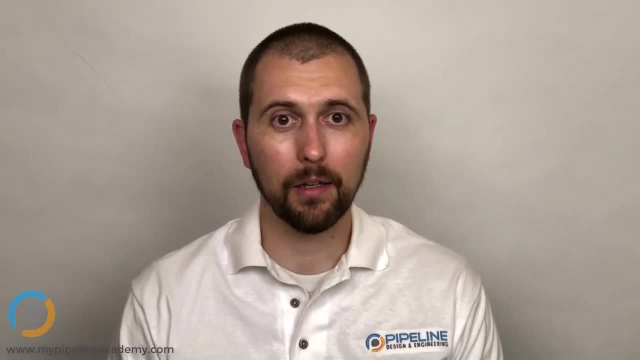 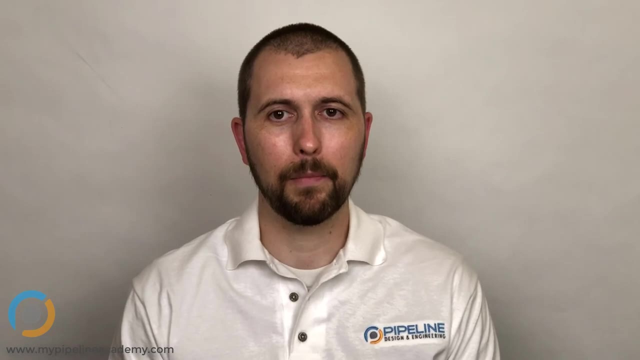 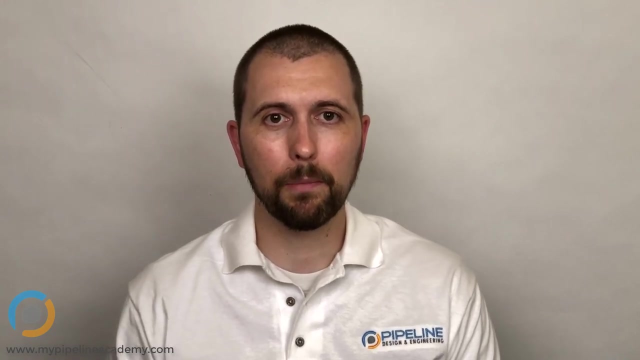 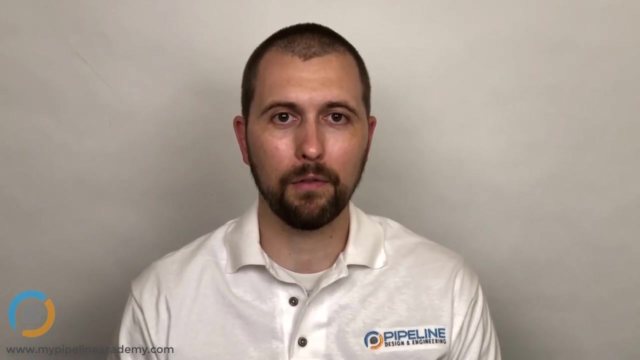 assuming your part geometries will accommodate grip pins, because not not all of them do. but assuming your part geometry will accommodate gripper pins, they're. they're a cheaper method of joining your parts and it is a permanent joining. once your gripper pins are set one side into the other, they won't come apart. uh, those pins themselves will will break off of the. 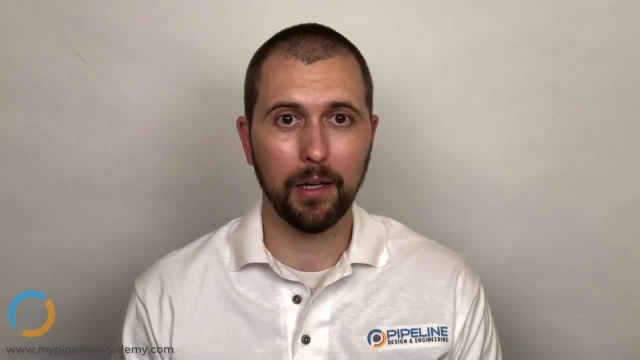 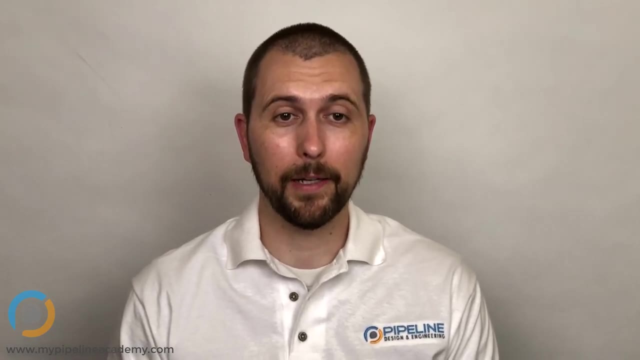 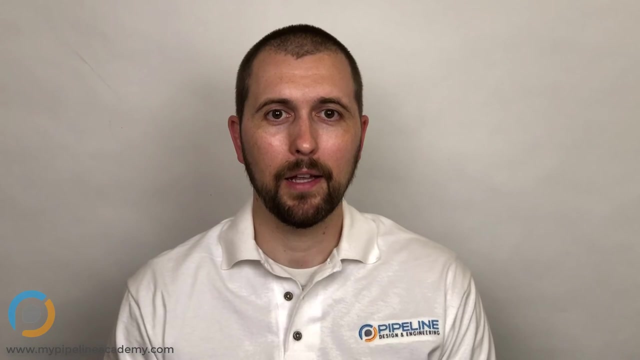 part before the interface between, uh the the pin and, uh the hole in which it's pressed will will fail. so they won't come apart. if they're done correctly, that's correct. yeah, and that is. that is one of the downsides to gripper pins, is they're? they're kind of tricky to get right and uh, not all. 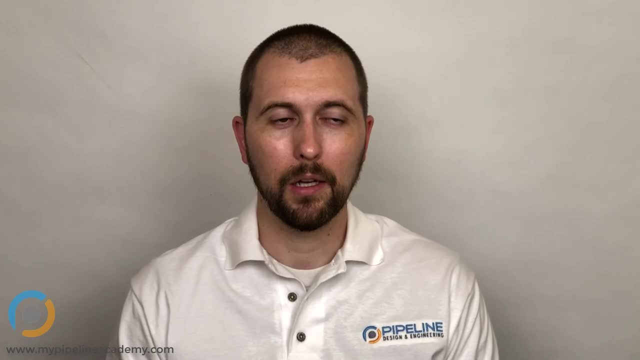 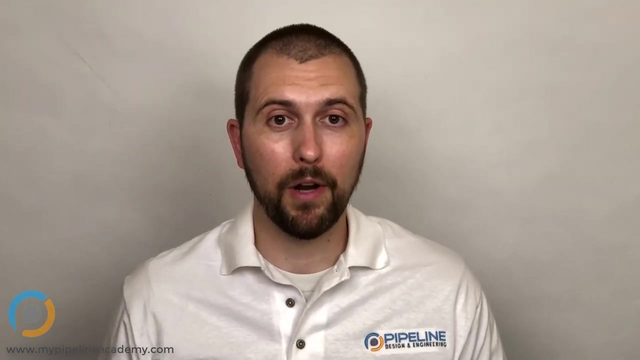 molders have a lot of experience doing them- uh, doing them correctly. they rely on very tight tolerances and some tricky molding practices. um, zero draft is is one of them. whenever you're injection molding a plastic part, you- uh you want to put draft on it and we get into the details of. 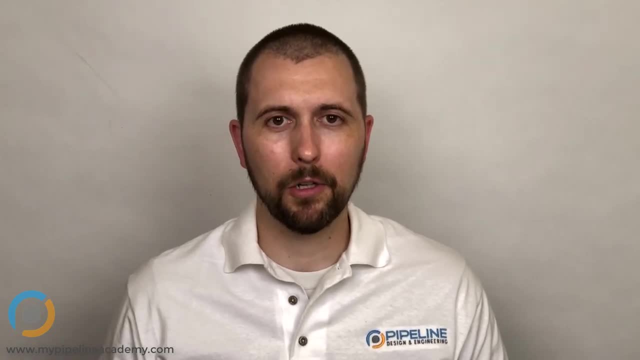 that more in some other videos and written literature. but, um, gripper pins, you want to have zero draft and that's tricky to do correctly. uh, a lot of our models um, have structure where they're of molders. don't have experience doing that so, yeah, that's another thing to.